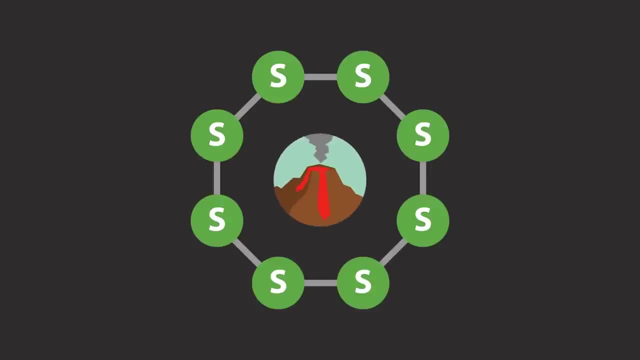 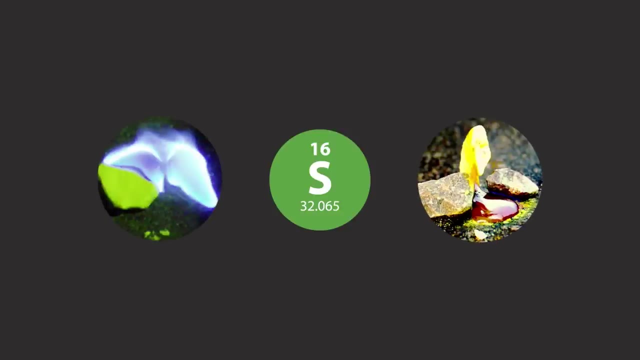 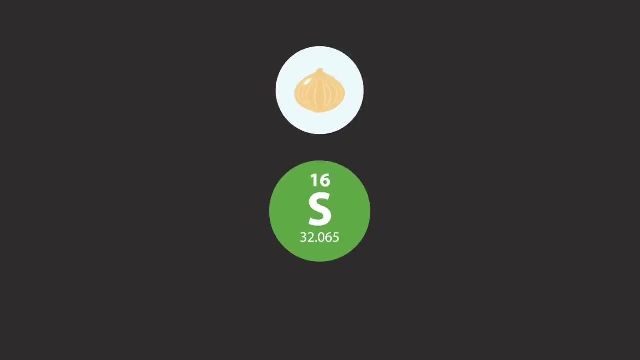 very prevalent in nature. It is commonly found around volcanoes. Yellow elemental sulfur burns with a blue flame and melts into a deep red liquid. Its many compounds can be found in everyday life. Does cutting onions reduce you to tears? The sulfur-containing compound responsible. 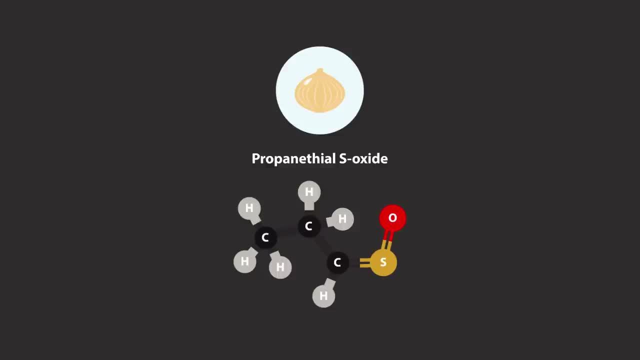 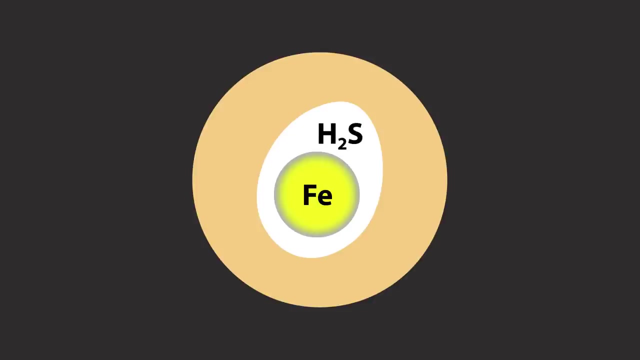 for this is a known substance that makes your eyes produce tears, Stinky feet and bad breath. Blame those on sulfur-containing compounds. too Overcooked those boiled eggs. That blue-gray lining around the yolk is due to the reaction of the iron in the yolk and hydrogen sulfide. 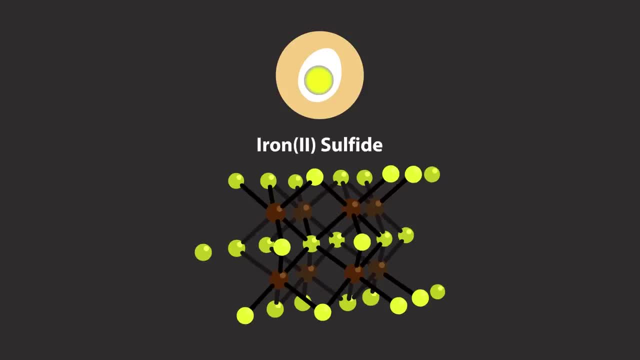 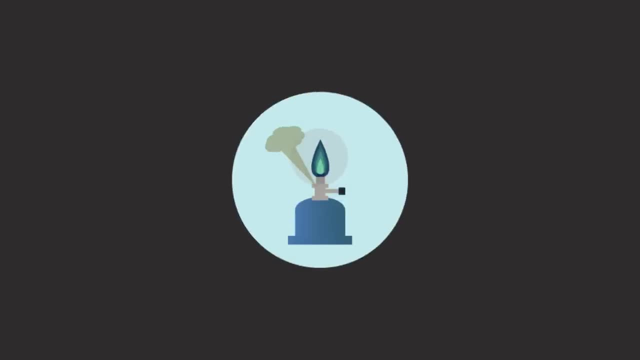 created in the whites forming iron sulfide, Ever smelled a natural gas leak? That is a natural gas leak. That is actually the smell of a spiking agent, which is a class of sulfur-containing compound called thiols or mercaptans, such as methen, thiol. Methane is the gas, the thiol is the. 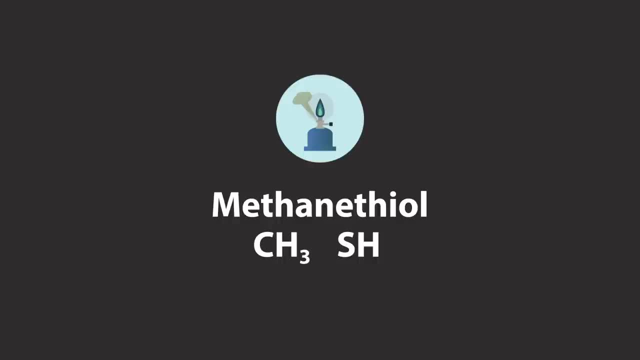 sulfur-smelling part. The sulfur smell is strong enough so that you can detect a potentially dangerous leak. In fact, fuel for cars and other vehicles also contain these sulfur compounds. The combustion of these fuels also means the combustion of these sulfur-containing compounds. 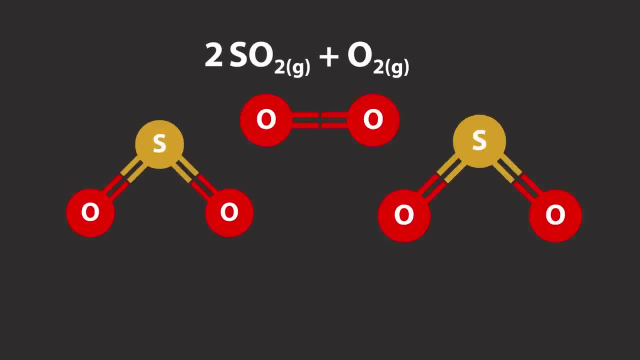 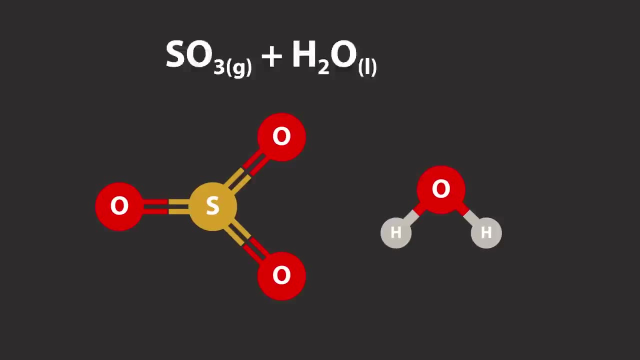 This results in the production of sulfur dioxide, Sulfur dioxide, which reacts with the oxygen in the air to create sulfur trioxide. Sulfur trioxide then reacts with water vapor in the atmosphere to produce sulfuric acid, Sulfuric. 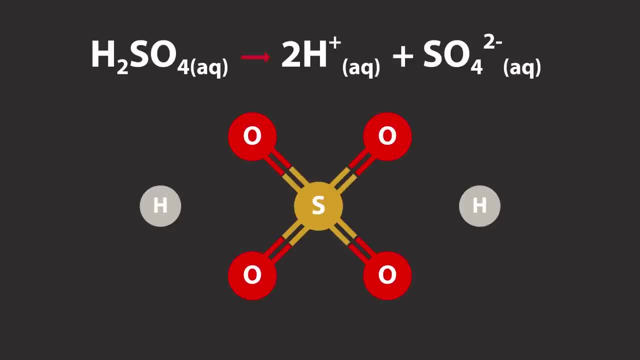 acid then dissociates into its respective ions, meaning there is a higher concentration of hydrogen in our rainwater and so the pH is lower. This means that it is acidic. Bicycle and car tires would not exist without sulfur. White latex is tapped from rubber trees In. 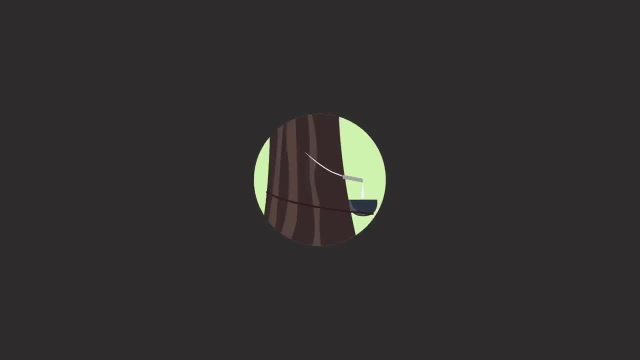 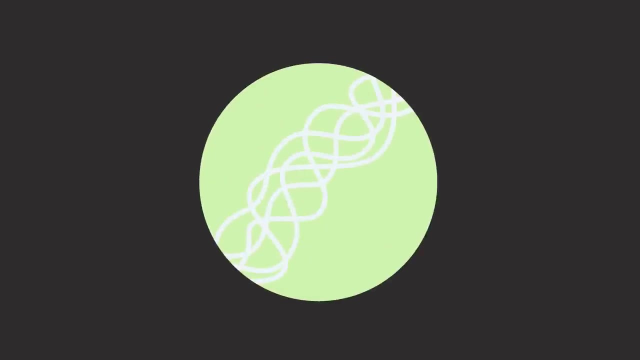 this natural state it is not very useful. so it is vulcanized or cooked with sulfur to make it harder, stronger and longer lasting. In its natural state, the rubber molecules are long chains that are tangled up and only weakly linked. When it is vulcanized, the 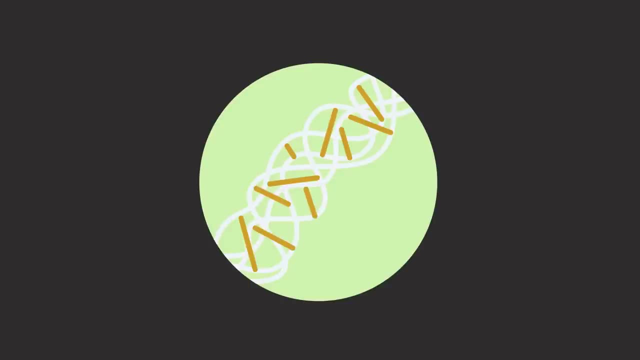 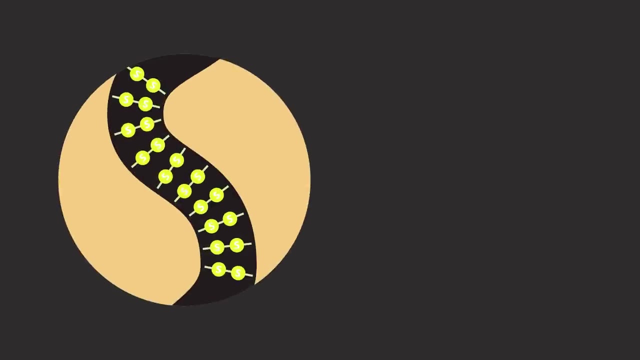 sulfur helps form extra bonds, which are known as cross-links. This makes it harder. Did you know that curly hair has a connection to sulfur? Keratin, the main protein component of hair, also has lots of disulfide bridges. The more